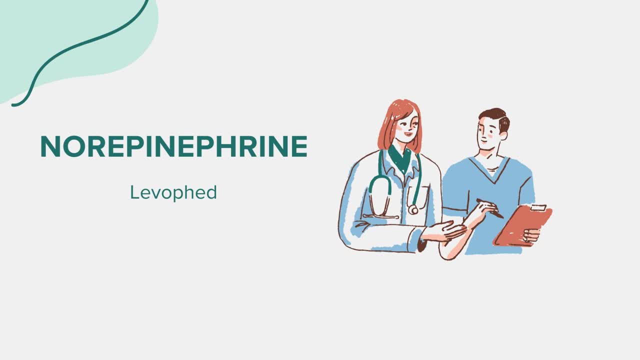 it's crucial to consult with a healthcare professional. Description: Norepinephrine, widely recognized under the brand name LevoFed, is a medication administered intravenously. It belongs to a class of drugs known as vasopressors, which work by constricting, narrowing the blood vessels, thereby increasing 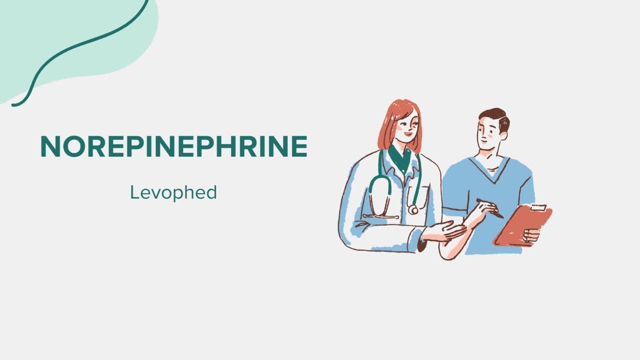 blood pressure and blood flow to vital organs. It is predominantly used in the treatment of acute hypotension, severe low blood pressure, especially when the condition is not responsive to fluid replacement. Norepinephrine is vital in managing shock, including septic shock. 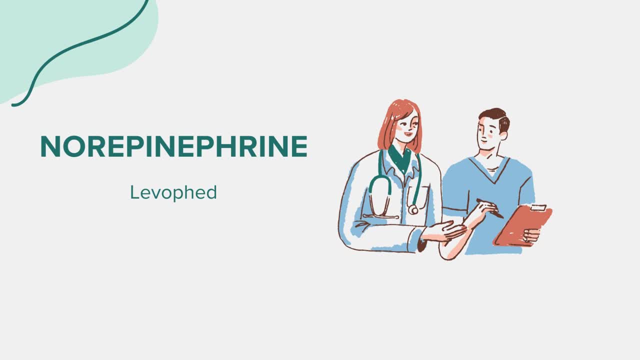 cardiogenic shock and other forms of distributive shock by stabilizing hemodynamics and ensuring adequate organ perfusion. Warnings: The use of norepinephrine requires close monitoring due to its potent effects on the cardiovascular system. It is contraindicated in patients with hypersensitivity to the drug and 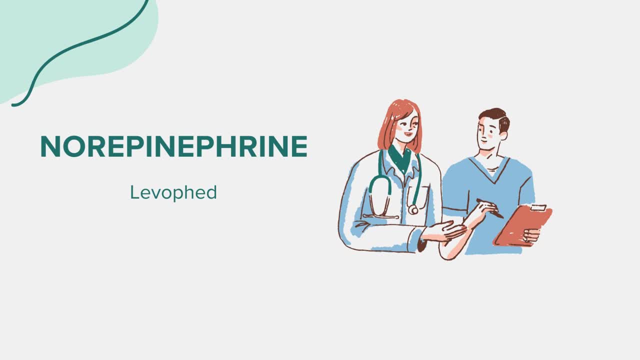 in situations where the administration could exacerbate conditions like thyrotoxicosis or certain types of tachyarrhythmias. Care should also be taken in patients with ischemic heart disease or chronic hypertension, as the increase in blood pressure could lead to adverse. 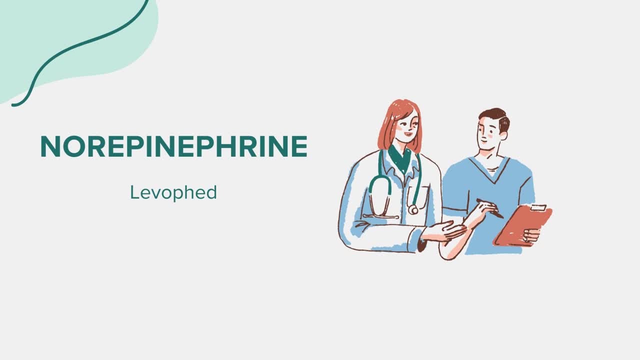 events Before taking this medicine. Before the administration of norepinephrine, comprehensive medical history and assessment should be conducted. This includes evaluating for conditions such as peripheral vascular thrombosis, as norepinephrine can exacerbate ischemia due to its vasoconstrictive action. Inform your health care provider if you have. 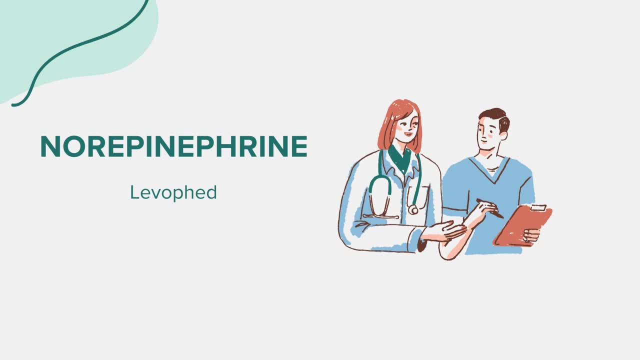 a history of hypertension, heart disease, diabetes or hyperthyroidism. Pregnant or breastfeeding individuals must discuss the potential risks and benefits with their health care provider. Side Effects: The administration of norepinephrine can lead to various side effects. 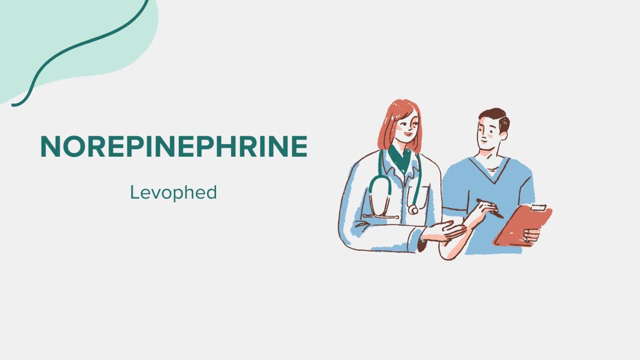 reflecting its potent pharmacological action. Common side effects include headaches, restlessness and palpitations. More serious adverse effects may involve cardiac arrhythmias, excessive hypertension and peripheral ischemia, which can lead to tissue necrosis. if extravasation occurs, Immediate medical attention is necessary if patients experience severe side effects such